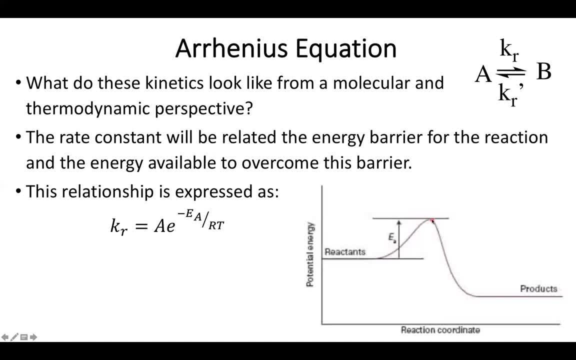 can get to this height of the barrier And again divided by a temperature factor, The higher the temperature, the more energy I'm going to have to pass over this barrier, And so this equational form is called the called the Arrhenius equation. 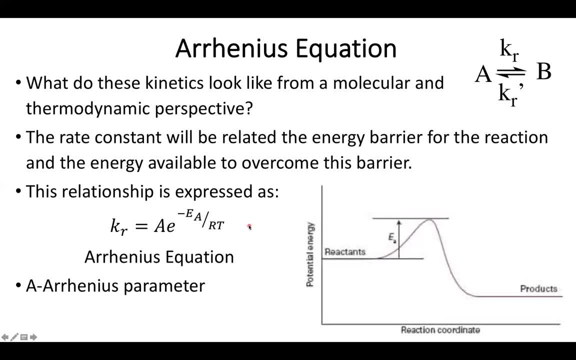 And so again, it's more or less just a special case of our Boltzmann form, With, again, focus here on the electronic energy and what's called the Arrhenius parameter. So it turns out that every single reaction is going to have a slightly different path. 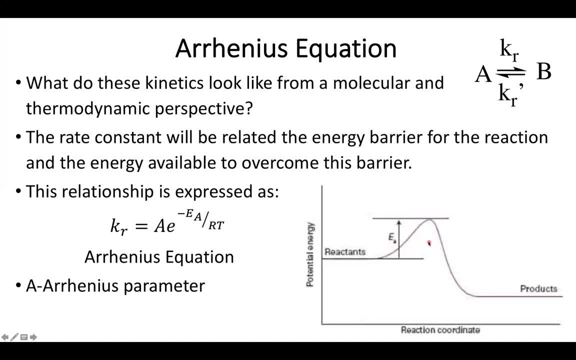 And so you can imagine, this Arrhenius parameter is going to be highly dependent upon, say, the shape of this barrier. It often will be, say, a much larger leading to much larger rates if I have a thinner barrier, which is going to be easier to get up. 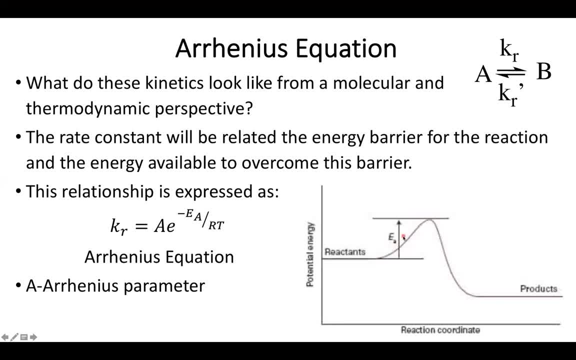 The lower the slope, the more time I have to try and spend climbing up and thus an effective, higher barrier. There's also important contributions in essentially the other dimensions of the reaction coordinate. Do I have to follow one single small path pathway through this mountain pass? 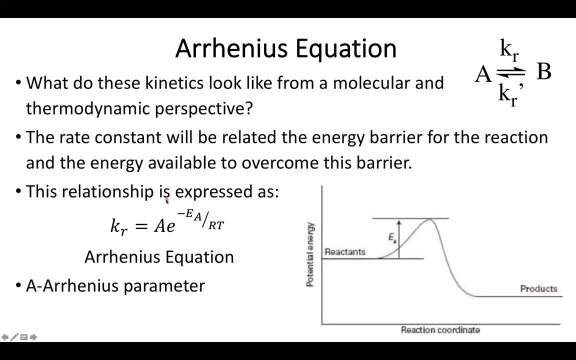 Or is there one single small pathway, or is there multiple different ways to get from reactants to products? All of this can highly influence the Arrhenius parameter, And thus it turns out that the Arrhenius parameter is going to have to be experimentally determined. 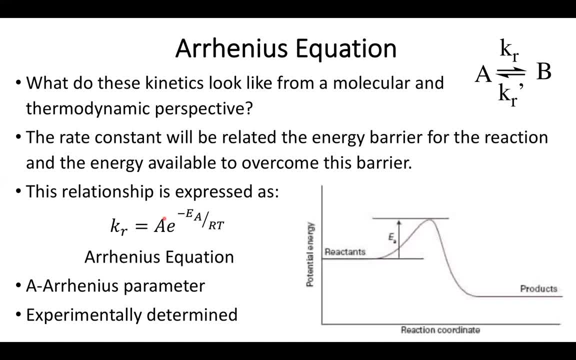 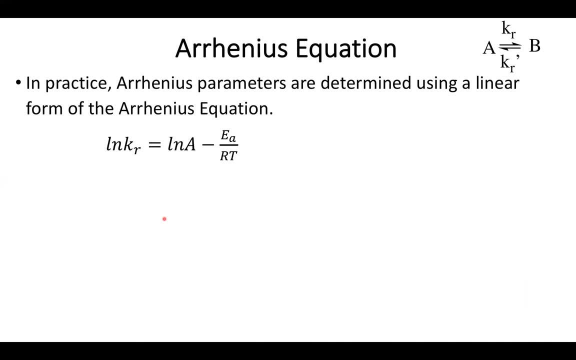 for every given interaction, So it's not like there is a one size fits all parameter, which can be slightly inconvenient. So when trying to go ahead and apply our Arrhenius equation to a reaction system, one of the things that we're often going to do- 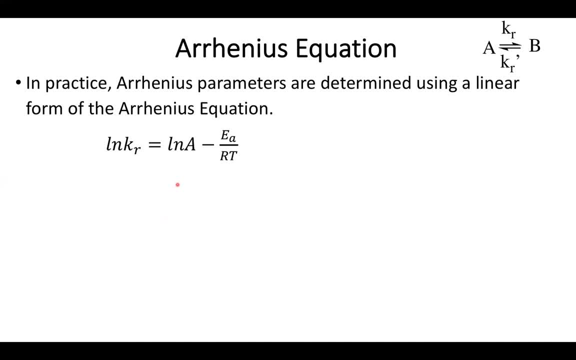 is trying to determine these parameters. We're going to do our good old favorite and see if we can fit the system to a linear equation. So the classic form of the linear equation we're going to do is essentially just taking the natural log of both sides. 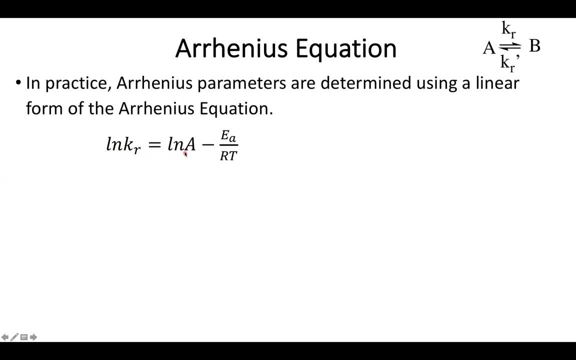 And we can fit it to natural log of the rate. constant equals natural log of the Arrhenius parameter minus activation energy over RT. So that's what we're going to do. So I can essentially obtain my two variables, in this case the Arrhenius parameter and the activation energy. 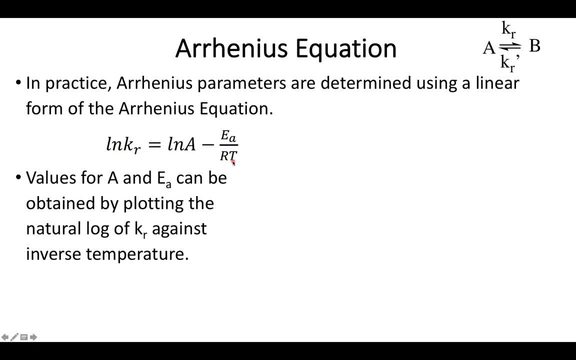 by plotting the natural log of the rate constant versus inverse temperature. And again, please note again that every reaction is going to have a unique set of variables, So you're going to need to do this to examine the rate of reaction for any given reaction. 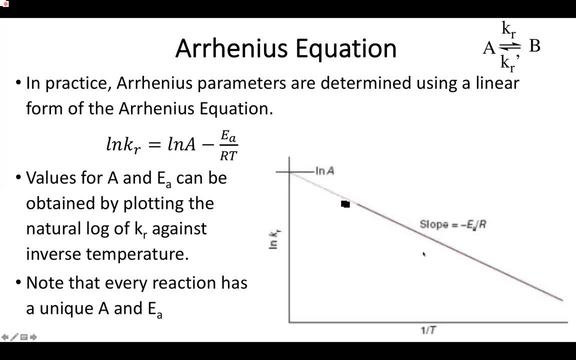 of interest. But again, the general idea is that the rate of reaction is: by plotting 1 over t versus ln of k, I should be able to pop out my activation barrier. But again, make sure to note that this equational form predominantly supposes that we are going to. 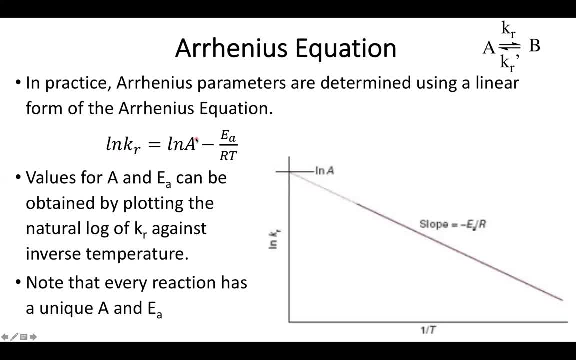 be making use of a reaction per second. However, any sort of choice of units on the rate constant will help be embodied in the Arrhenius parameter, which will have the same units as our rate constant. So again, one of those things to kind of keep an eye out for. But again, this equational 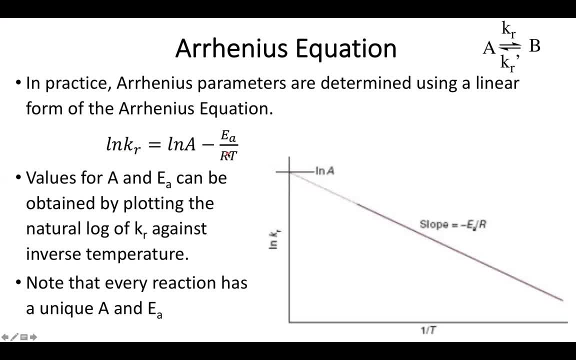 form is making use of our activation energy, And this isn't exactly a thermodynamic property that we've really seen too much, because this is an electronic energy. It only depends upon the electric field, So this is an electronic energy surface which is inherently just a little bit too much quantum. 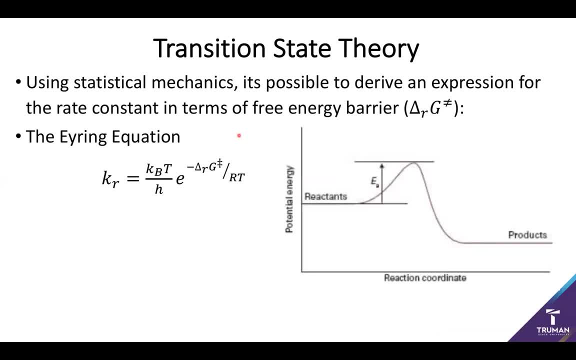 for us right now. However, it's entirely possible to apply statistical mechanics to this system in order to derive an expression for a rate constant in terms of our free energy barrier, which I'm going to call delta G double dagger, And so it's essentially the free energy. 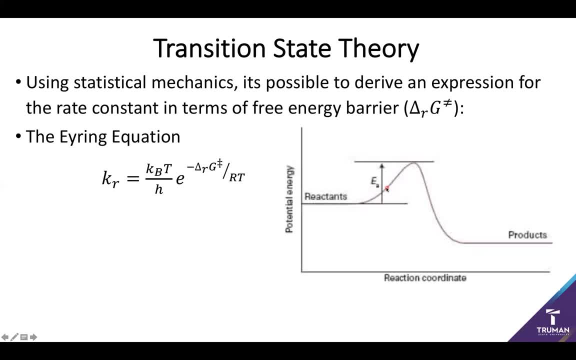 equivalent of the Arrhenius equation. So this is going to be our activation energy, Except for now, instead of just being in terms of the electronic energy barrier, it's now a full energy barrier. So this is in counting enthalpy and entropic contributions, And it's going to be- and it shows the rate- constant to. 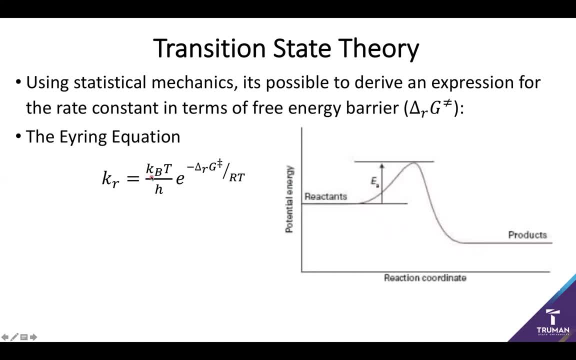 be dependent upon the Boltzmann's constant, our good old friend, which isn't too surprising as this is a general Boltzmann's form. So this is the state of our chemical reaction. So the temperature is the direct energy of the system. So this is the temperature of the system and the Planck's constant, which is the first. 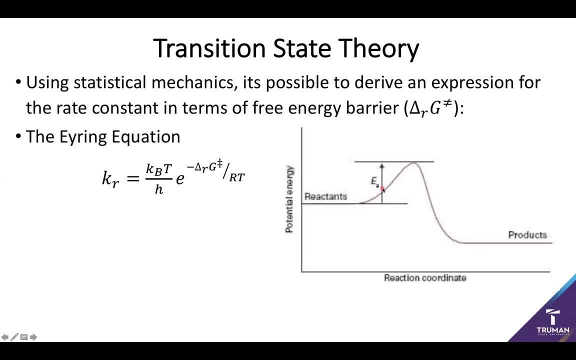 time we've been seeing this constant this year, but we'll see it pop up more and more the more quantum mechanical our systems become. and again, our free energy barrier of the reaction And again, one of the things I want is really just the free energy of our transition state with respect to the reactants And a good 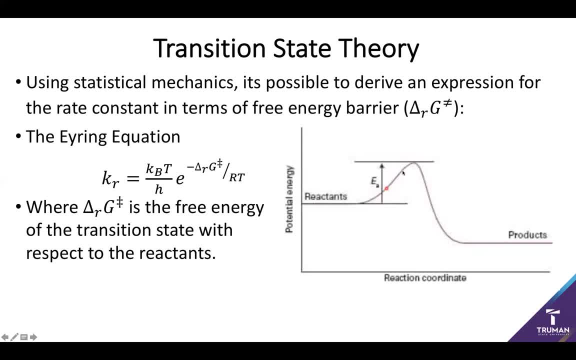 way to try and look at these transition states is to think of them as the highest energetic point on the potential energy surface. So essentially, if I'm trying to go from reactants to products, I'm being channeled past this single point And again, what matters is less the arbitrary. 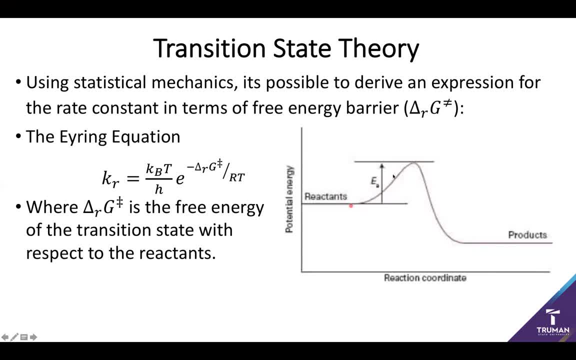 free energy point, but more the difference of where I started to where I have to get to. And one of the other things that I really want to go ahead and point out here is going to be the units on this fun little pre-factor of Boltzmann's temperature and Planck's, Because 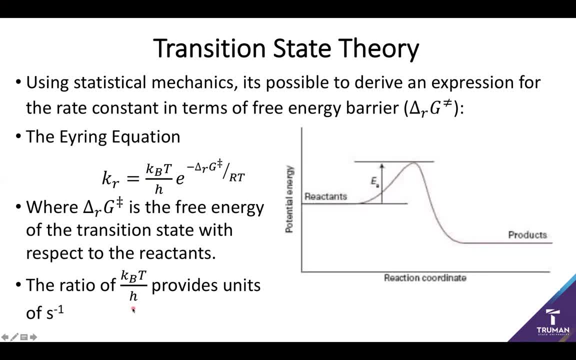 it turns out, when you actually run the units for these three variables, it turns out that they provide units of per second. So the reason why we have units of per second here is because, you may notice, those are the same units of a first-order rate constant. 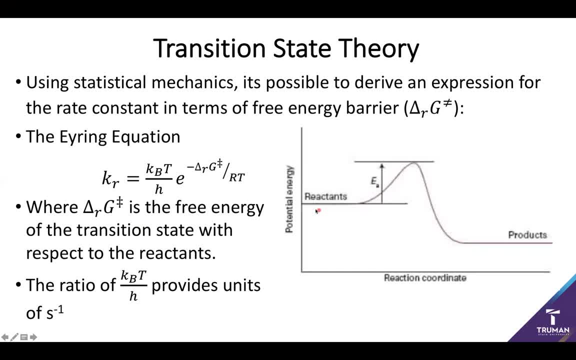 So, intrinsically, what we are doing is we're assuming that all of our reactants are part of one single pre-reactive system. So, as a result, any sort of rate constant is going to be the same unit of a first-order rate constant. 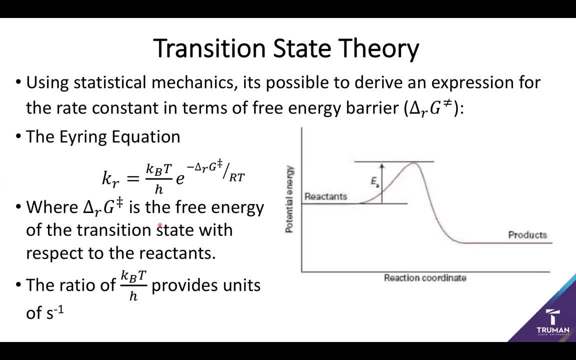 So we're assuming that all of our reactants are part of one single pre-reactive system. So, as a result, any sort of rate constant determined from the Eyring equation is going to have to be first-order in nature, as it's going to neglect any energy of the reactants themselves coming together. It's assuming them as 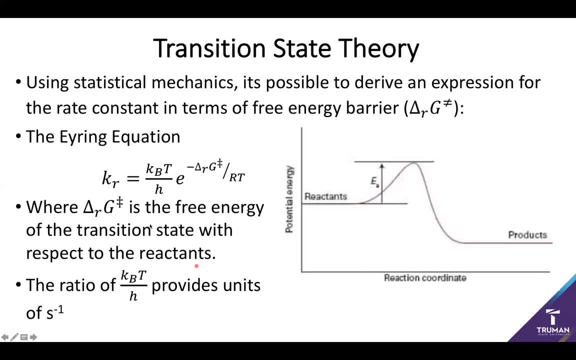 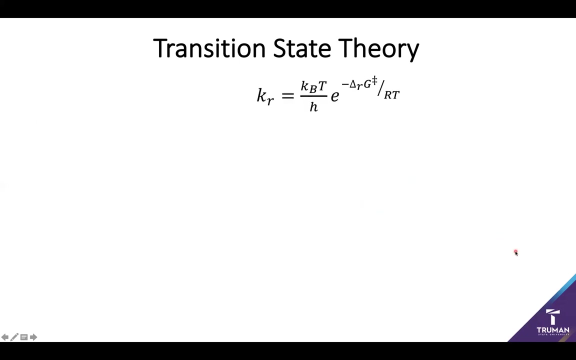 one collective unit. However, it is possible to essentially use this rate constant to essentially emulate first-order or pseudo-first-order rate kinetics, So this can be a useful construct. nonetheless, And again using this, we can essentially develop a pseudo-first-order rate constant for progression of reactants to products, which will then help us describe the real reaction rate of the system. 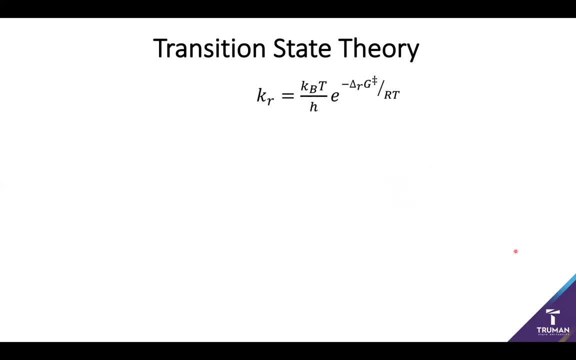 However, one of the things that is also fairly useful to do is to try and break our Eyring equation down into thermodynamic components that we may be a little bit more familiar with. So our classic choice here is trying to break it into the N-type. 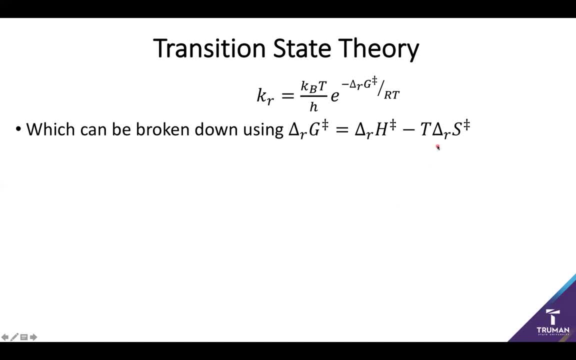 The N-type is an enthalpy and entropy of activation, And doing this I can substitute in my equation for the free energy of activation into the Eyring equation. And so now we break the term into an exponential expression, into a negative delta h over RT and a positive entropy over R, where essentially, if you notice here, the negative signs and the two temperature terms should end up canceling out. 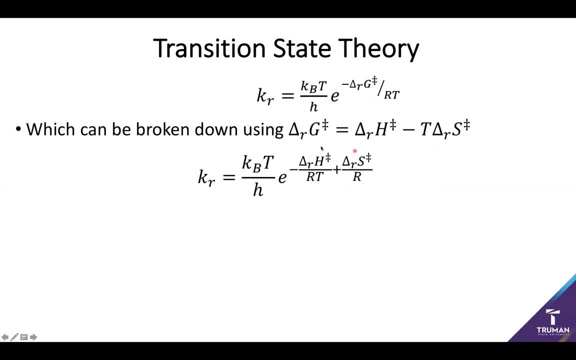 However, this becomes a rather long exponential expression. So, using our good old exponential rules, we can also break this up into the product of two smaller exponential groups. So again from here we can predict the rate constant based on a temperature-dependent term. 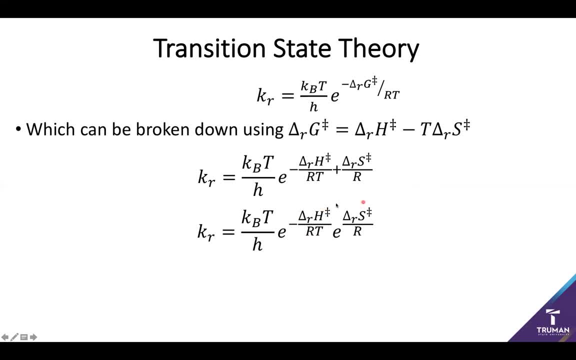 an enthalpy-dependent term and an entropy-dependent term Now, because sometimes it's more useful to deal with equations that do not show exponential behavior. one classic choice is to remove the temperature dependency over to the left-hand side, leaving together just a set of. 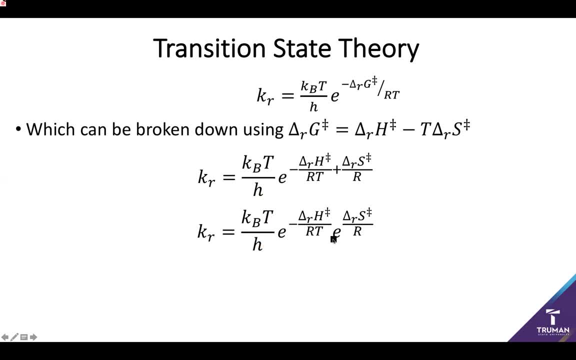 constants out front and then taking the natural log of everything to get rid of those exponents. This reduces the system into a natural log of a rate constant over temperature, a natural log of two constants: an enthalpy-dependent term and an entropy-dependent term. 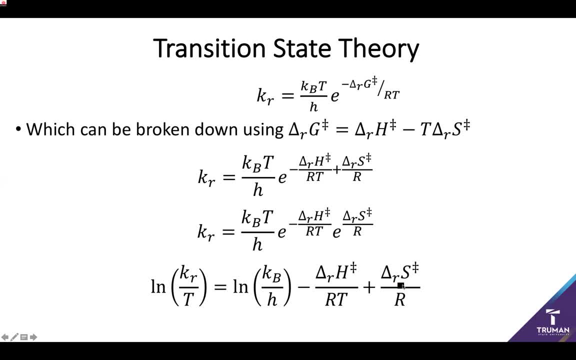 And one of the reasons why we specifically like making use of this form is that you may notice that this has a general linear relationship sort of form where our major unknown here is going to be the temperature dependence. So it's possible that you can measure. 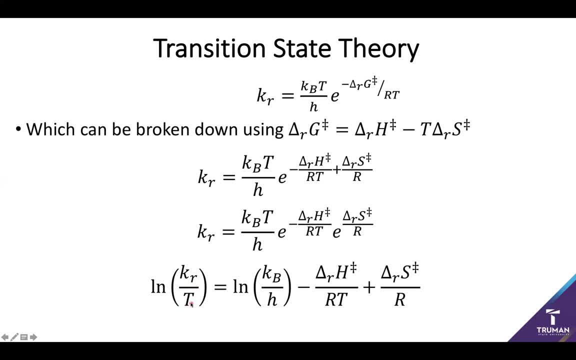 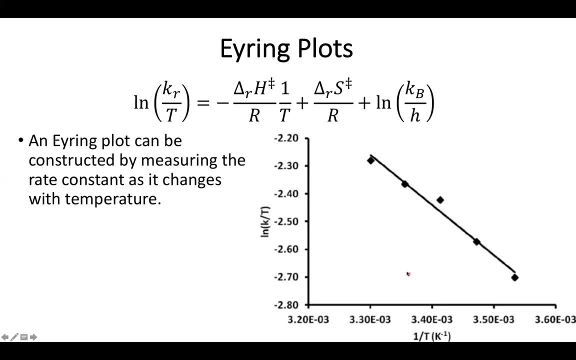 your temperature dependence by taking the natural log of everything to the left-hand side- your rate constant at multiple different temperatures- in order to be able to extract that information about the enthalpy and entropy of activation. So in this case we're going to 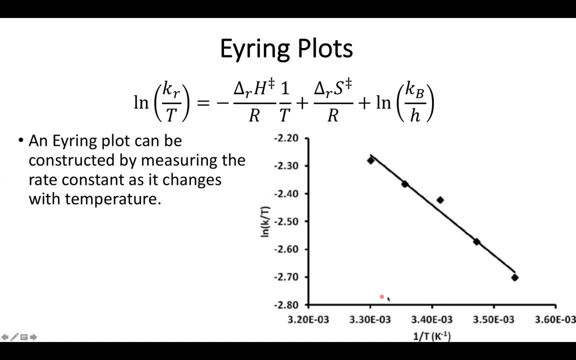 plot natural log of the rate constant over T versus inverse temperature and essentially measure how our rate constant changes with temperature And doing this we're able to essentially obtain the enthalpy of the transition state, again with respect to our reactants. 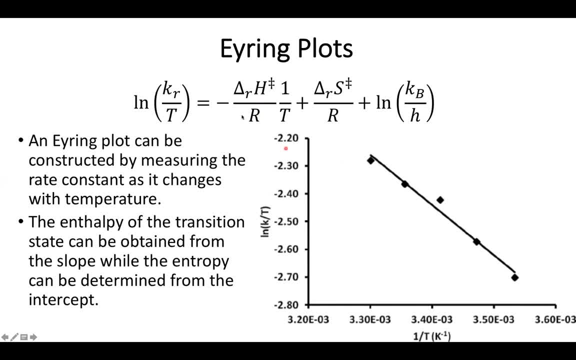 from the slope of the equation, as the slope should be negative. delta H over R, while our intercept is going to be these last two terms and is going to provide us information about the entropy of the transition state, as well as embodying these two constants. However, one of the things 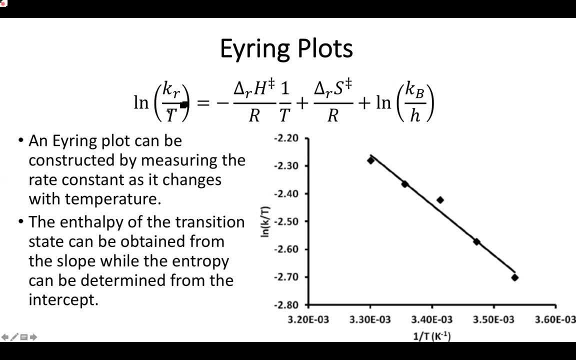 that is important to note is: please make sure, when you do this, that you're making use of your rate constant in a per-second notation. Otherwise, any unit conversion will actually also be embedded in this intercept and can throw off any potential measurement values. So because of this sort of subject to units and other choices, 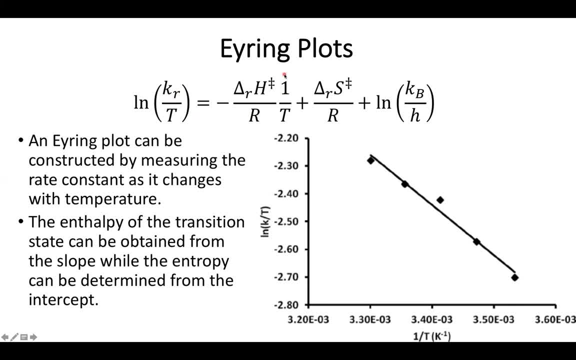 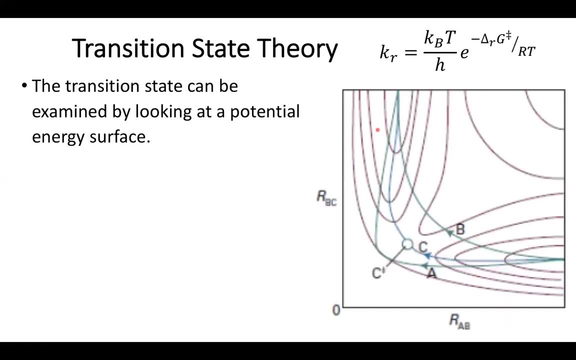 it's not uncommon for the enthalpy of activation from an iron plot to be fairly accurate, while there may often be severe inaccuracy coming from the entropy. Now let's go ahead and try and examine a little bit more about what these components really kind of mean, And so you can actually get some of this. 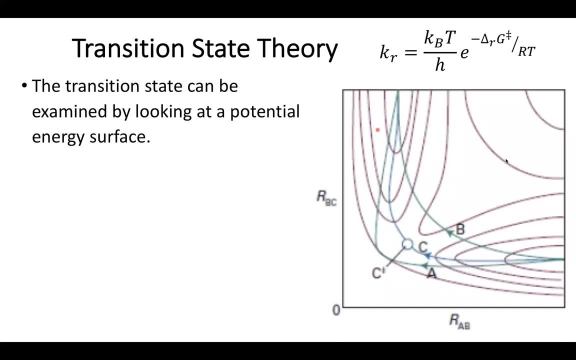 meaning by looking at the potential energy surface. So if I have a reaction, really what I'm trying to do is I'm trying to start from a reactant pool and go to a product, And this is often going to be involved in some sort of bond forming, which we're showing here as the distance of atoms A and B. 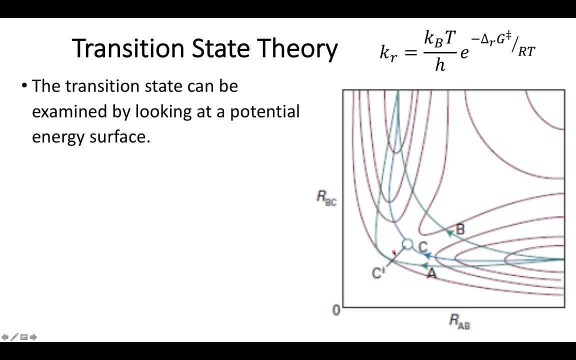 decreases And a bond breaking, as we're demonstrating, with distances of bonds B and C elongating, And so when you do this, you often reach some crucial, crucial point, where I've reached this high point in the transition state. So, really, what I'm seeing, 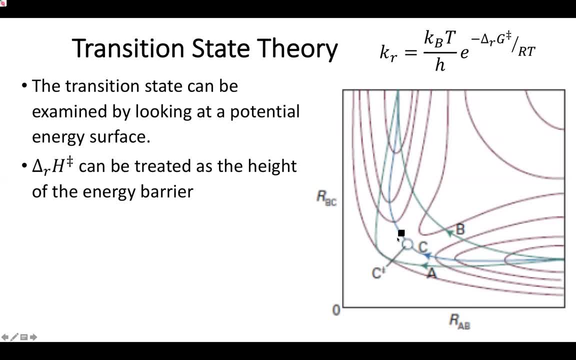 when I'm looking at, the enthalpy of activation is essentially the height of this barrier. So this differs slightly from the electronic energy due to a couple of quantum mechanical features involving vibrations that we'll talk a little bit more about next semester. However, one of the other 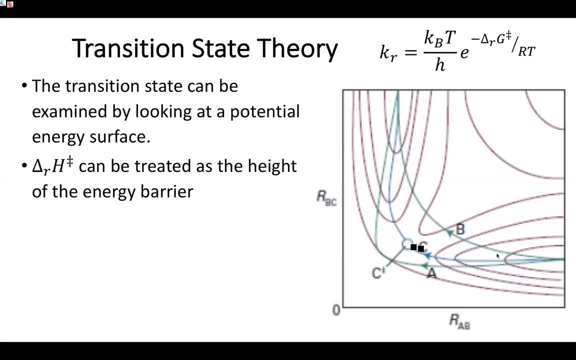 important components is that the difficulty to pass this barrier is also going to be highly dependent on whether I have to stick strictly to this lowest energy path, or are there enough energy states, tightly enough packed, that I can say: sneak a little bit to the side, cut a corner? 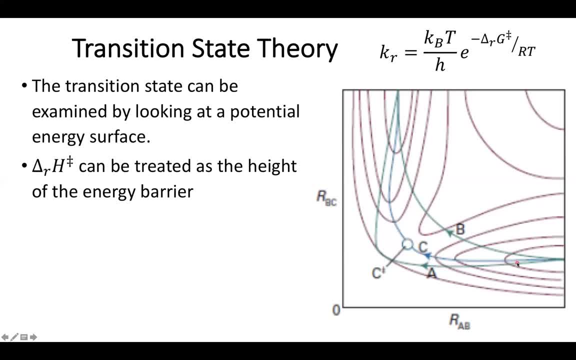 Because even while this might be the lowest energy path, be the lowest energy if this other path isn't too much iron energy but there's more of them, I'm going to be much more likely to pass by this transition state. And it turns out this is pretty. 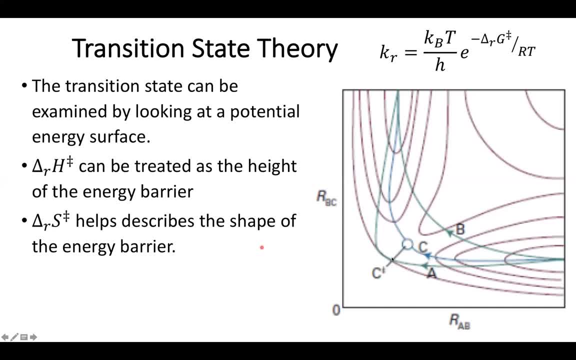 much kind of the definition of our entropy of activation. Essentially, do I have a tighter? is my molecular forms more tightly constrained in my reactant basin or at the transition state? If I have more places I can be in the reactant than at the transition state, this will tend to 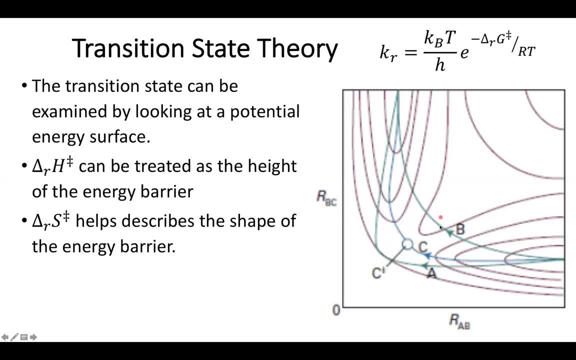 be unfavored. However, if I have a fairly wide reaction path, we'd expect to find a very positive entropy of activation. So, again, these are one of the things you should keep an eye out for. And again, what we're seeing here is generally a low energy barrier is going a low energy barrier. 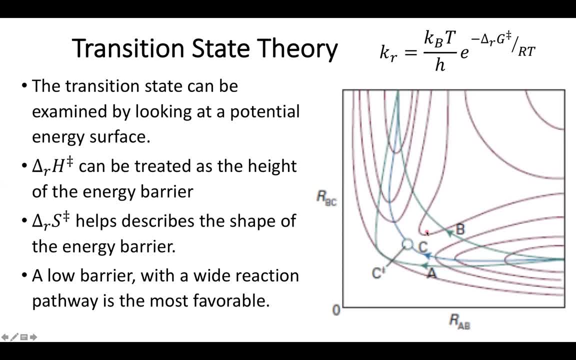 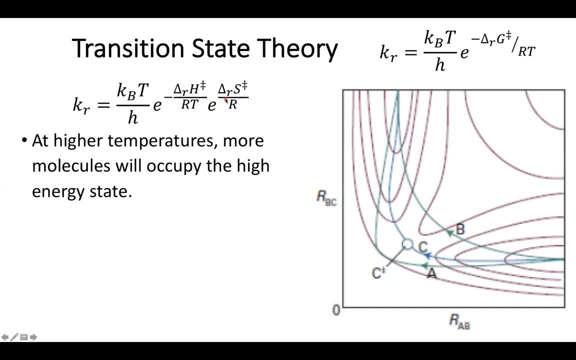 with a wide reaction path Is going to tend to be the most favorable. However, I also want to tend to look a little bit more at each of these components independently. So one of the first things I want to kind of emphasize is that, at higher temperatures, what I've done is I've essentially given the system 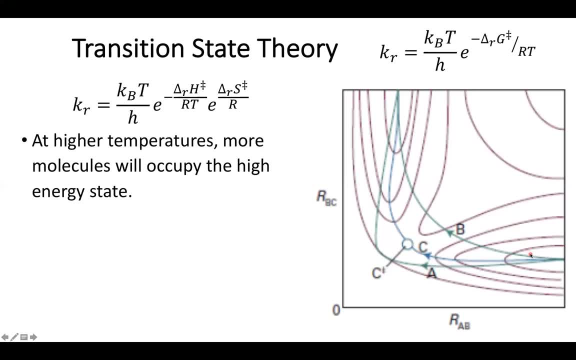 more the system in the reactant state is more likely to be found at higher and higher points, as we've seen before with Boltzmann. The more energy I have, the more likely I am to occupy an elevated electronic state. And as I'm occupying these, 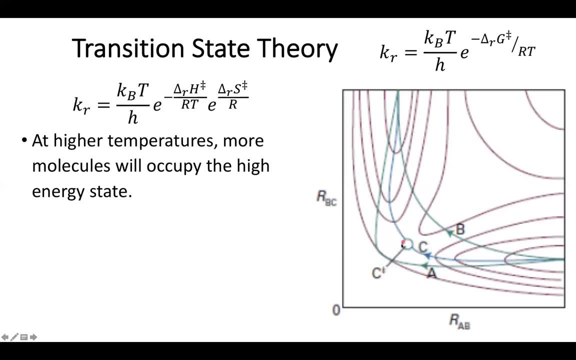 higher electronic states. it's going to make it much easier for me to pass by this saddle point demonstrated by the transition state. So this is one of the reasons why we'll tend to see at higher temperatures I'm reducing the effective barrier of reaction and making it easier to pass. 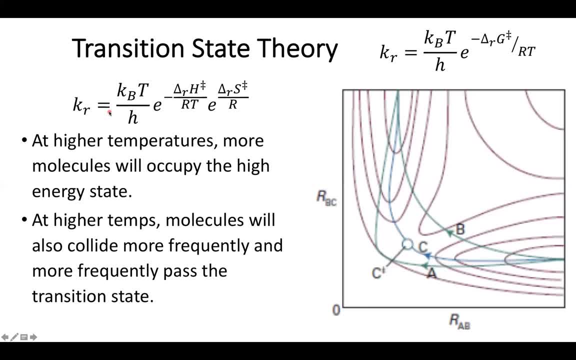 through and thus tend to have a higher rate, constant, Similar. at these higher temperatures, our molecules are also going to collide more frequently and they're going to have more energy to kind of pass through the system, which is really where this temperature expression of the pre-factor. 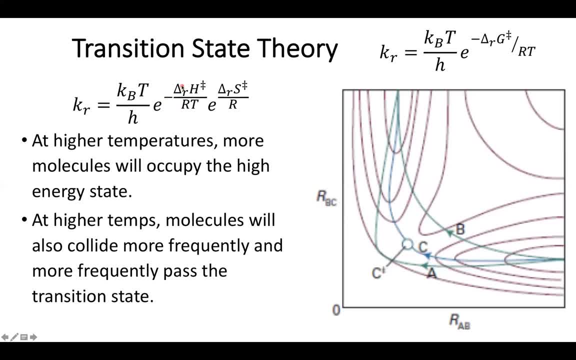 has. Whereas the temperature dependence on the enthalpy tells me how likely I am to be up here. the temperature dependence here says that if I'm up here, if I'm near the transition state, I have higher energy, I have higher movement. I'm much more likely to pass through. 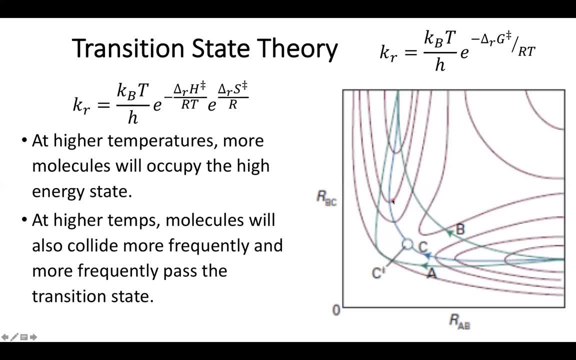 So, as a net result, one of the things that we tend to see is that, typically, when you increase the temperature of a reaction by, say, approximately 10 kcals, we tend to see an approximate doubling of the rate. Now, this is very dependent on the individual system you're examining and is going. 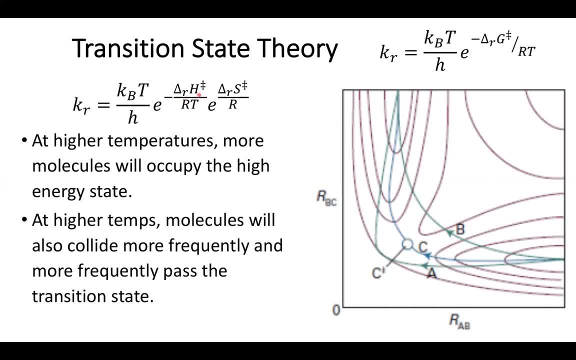 to be highly dependent upon the enthalpy of activation, but it's a good general rule of thumb. You increase the temperature by 10 degrees. you tend to see a doubling of the rate. Eventually, you have multiplied the waiting time by 10 degrees. This can mean that temperature 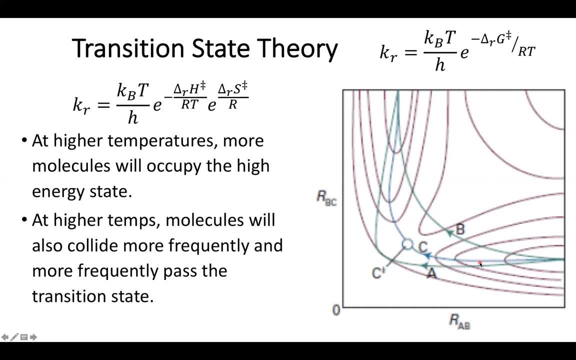 will be drying out, and so it's schedule-yani-vary instead of vir storytelling, Which can be very important to think about when you're thinking about the speeds of reaction, and it's one of the reasons why, in the real world, industrial chemists love to get their 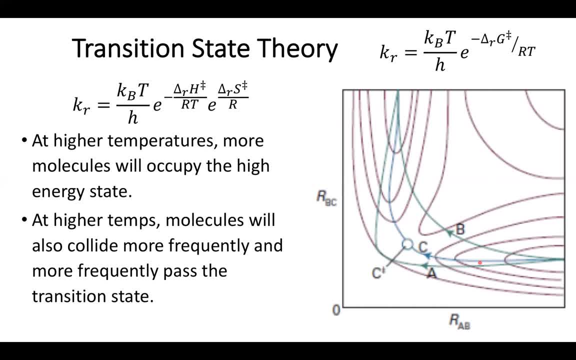 systems up to high heat, because then everything goes faster. That's also the reason they love catalysts, because that reduces the effective energy barrier. It reduces the effective energy barrier, However, depending on what you're krieg How do. It's also one of the reasons why biological systems love to also operate at high temperatures. why, say, warm-blooded animals are so favored? because at higher temperatures all of our metabolic activity goes so much faster. 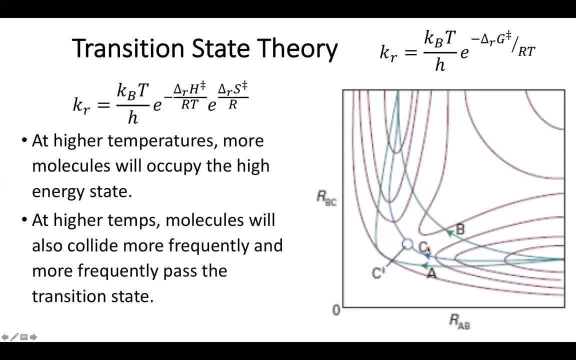 However, in biological systems we also have to watch out for unwanted biological activity to go so much faster, mostly degradation. This is why a fever can be painful, because you're actually going to help drive forward the reactions of decomposition of important amino acids and other protein groups. 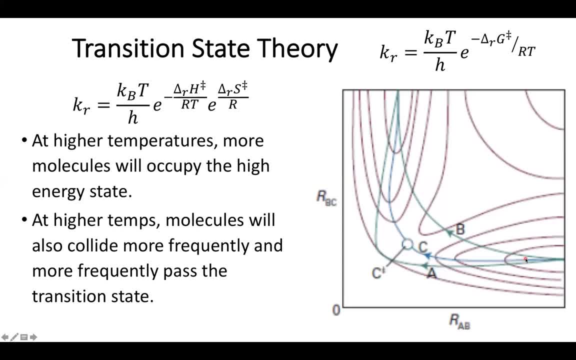 However, all of this has been strictly assuming that a reaction is proceeding unidirectionally from myeloma. So my reactant to my product and, most importantly, another important approximation of the ironing equation is: once I get to this point C, this transition state, I will automatically pass through to the other side. 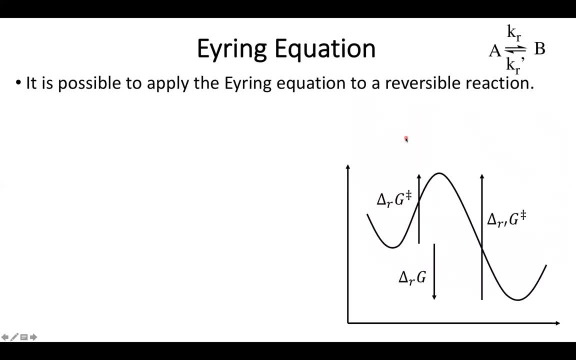 However, in reality the reactions do tend to go in reverse. So you can actually apply the ironing equation to the reverse reaction as well to see how the system moves forwards and backwards. So again, our forward reaction is going to be dependent on the free energy of activation for the forward direction and the reverse reaction is going to have a rate constant of the same general form but dependent on the free energy barrier of the reverse direction. 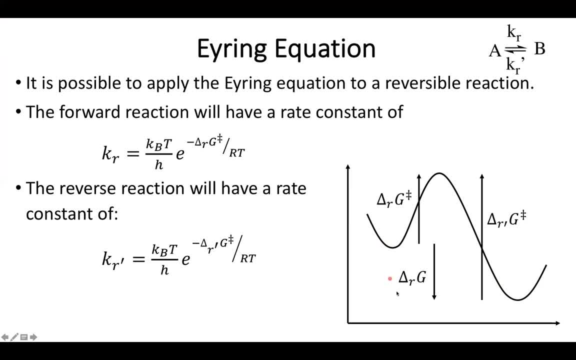 And again, these two energy barriers are going to differ by, essentially, the free energy of activation. Essentially, my transition state hasn't moved, but the minima that I start from has. So what we can do is try and use this to determine our equation. 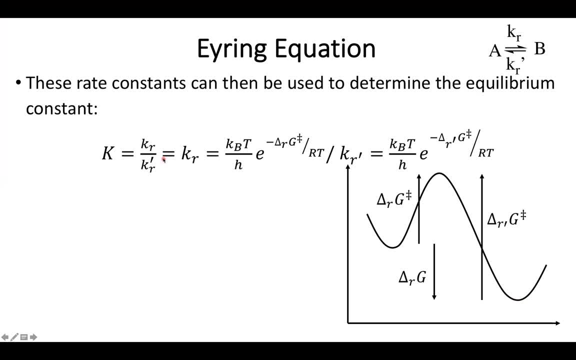 Equilibrium constant with the same equation we derived last time, where our rate constant for the forward direction divided by the reverse direction is going to essentially give me my equilibrium constant. Well, we can go ahead and plug in our two rate constants of forward and back and reverse directions and then essentially just take the ratio of these two forms.